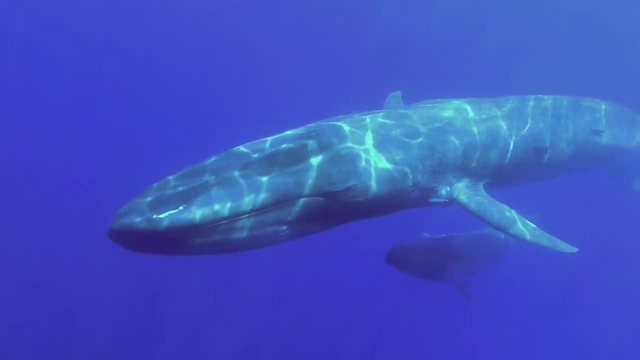 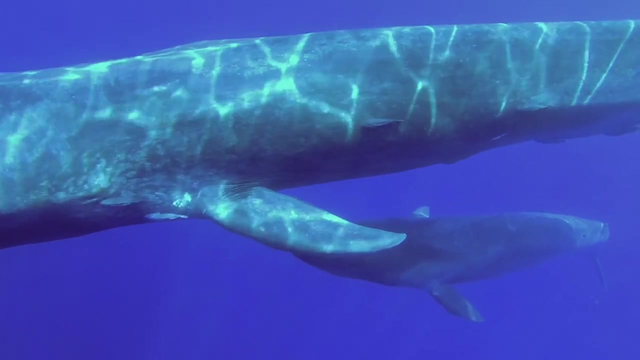 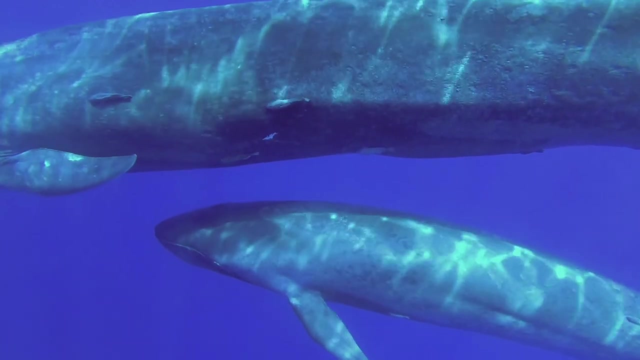 In summer, they feed on tiny krill in cool waters close to the north and south poles. In winter, blue whales are found in warm tropical waters near the Earth's equator. While whales must live in deep water, the members of our next kingdom plants are usually found in. 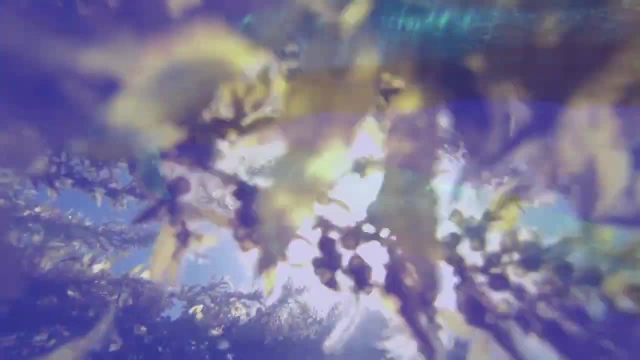 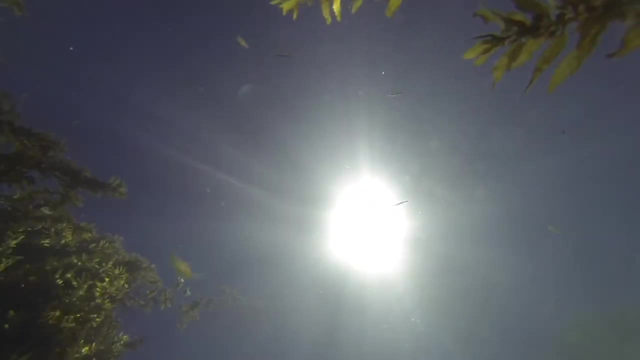 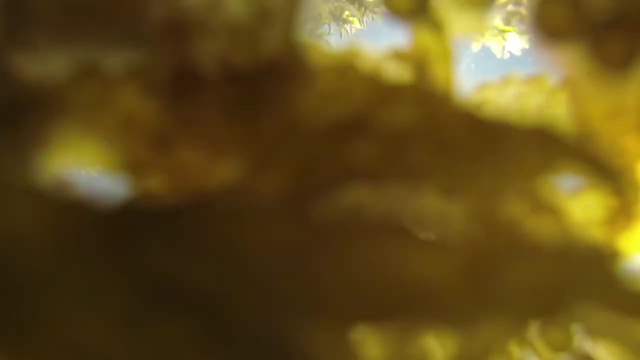 the ocean plants are usually found in shallow water. All marine plants need sunlight to survive. As a result, most marine plants live near the ocean's surface, where they can capture energy from the sun. Ocean plants have special adaptions that allow them to withstand salty waters and survive. 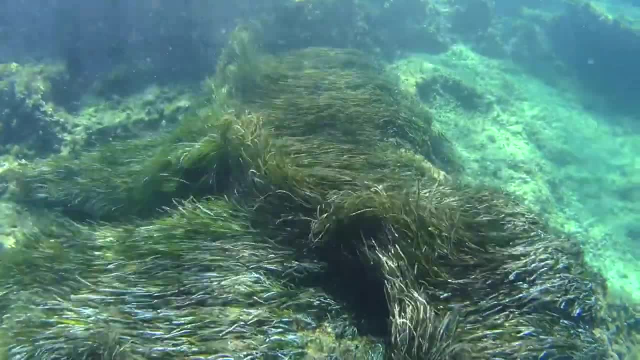 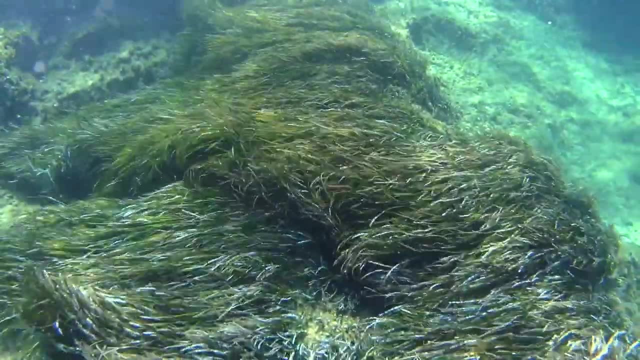 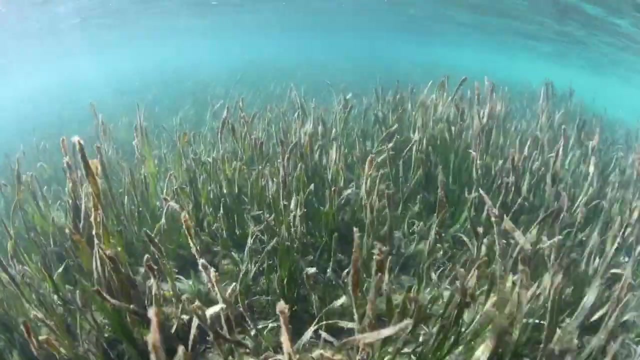 rough waves and strong currents. But like the plants that live on land, marine plants also have roots, leaves, flowers and seeds. More than 50 species of seagrasses grow in beds or large patches on shallow seafloors. 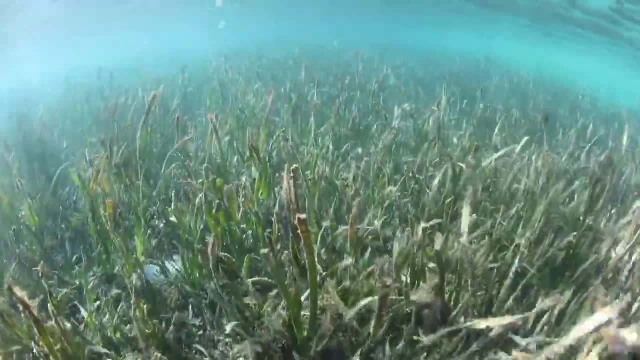 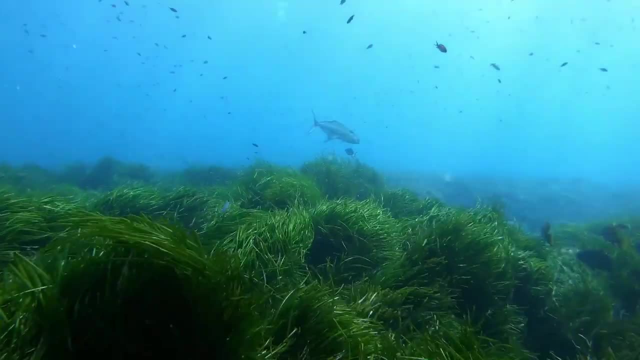 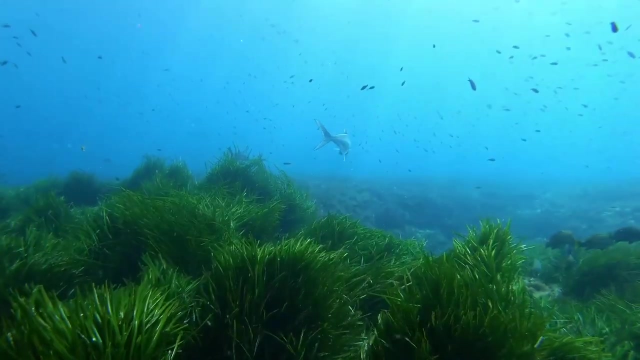 Sometimes they cover vast areas and are known as seagrass meadows, some so large they can be seen from space. The names of these plants are often used to describe marine plants: Seaweed plants, turtlegrass, surfgrass, paddlegrass, stargrass and more tell a story about their 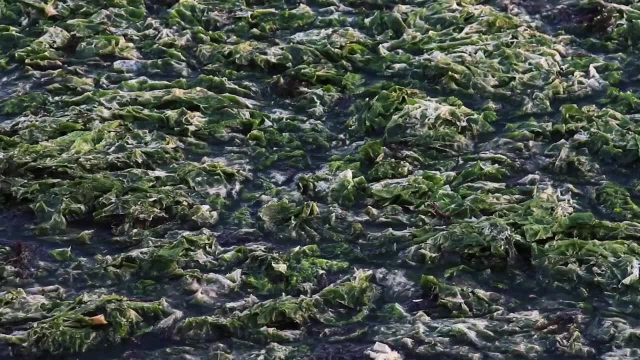 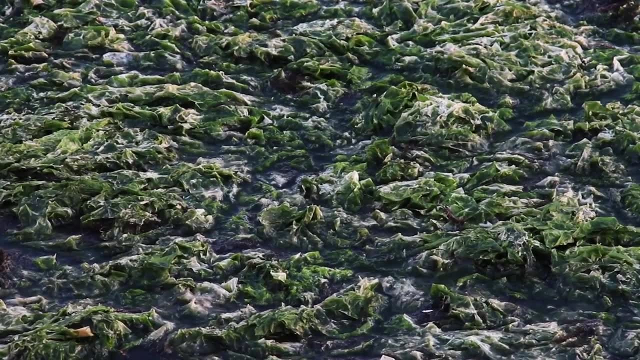 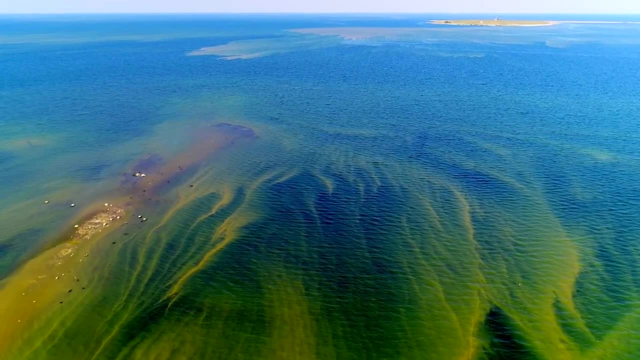 place within ocean habitats. Seaweeds are different from seagrasses. They are actually not plants at all. Seaweeds are algae, And algae are a large part of our next kingdom of marine life, called protists. They are a major part of our planet's marine ecosystem. 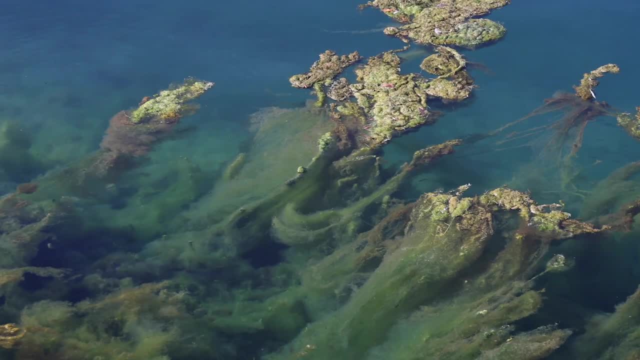 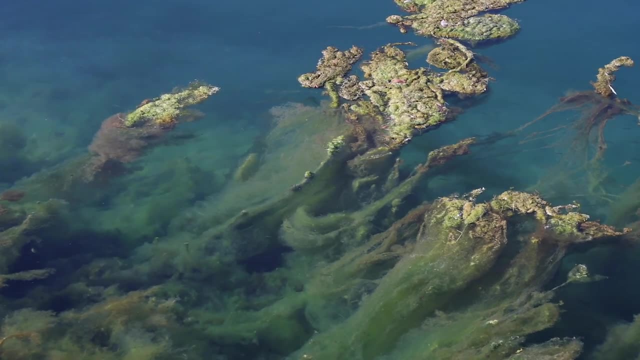 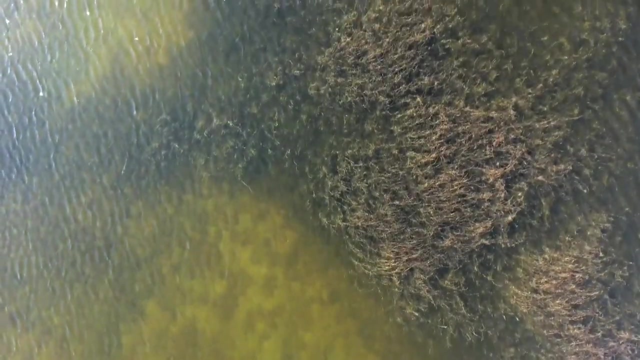 Many people consider algae as a natural substance. Consider algae with its slimy texture to be an annoyance, But algae plays an extremely important role in the ocean. Whether green, red or brown, algae is the main food source that almost all marine life 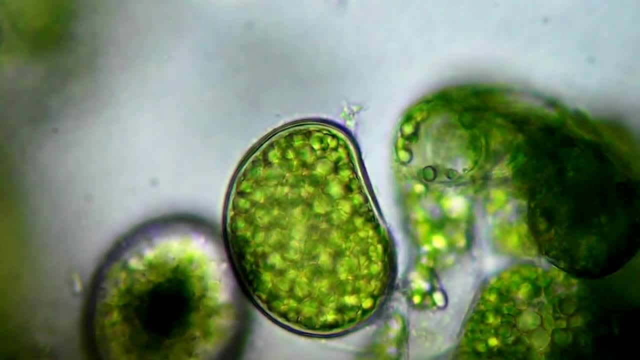 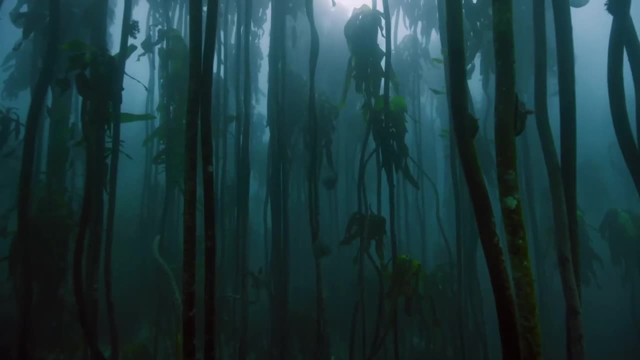 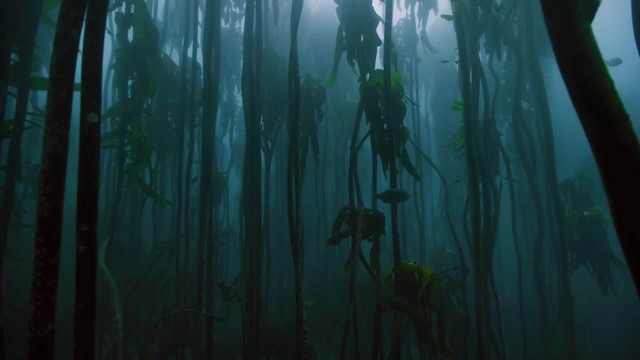 depends upon Algae can be small, such as the minuscule single-celled phytoplankton that drift in the seawater, or large, like the giant kelp that can form massive underwater kelp forests. Many marine creatures make their homes in these immense kelp forests, which provide